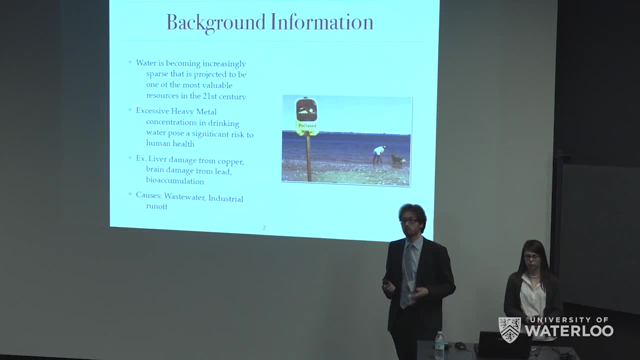 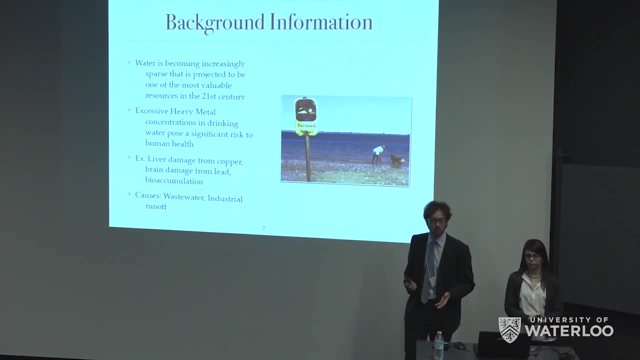 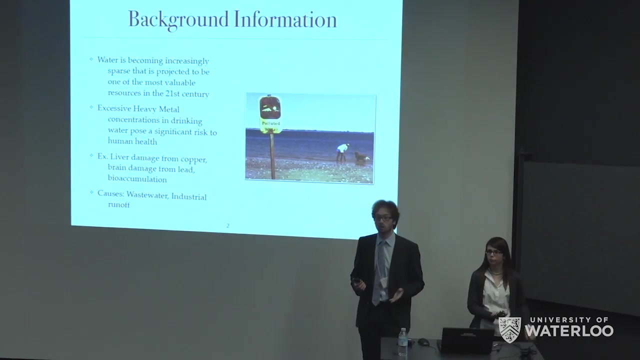 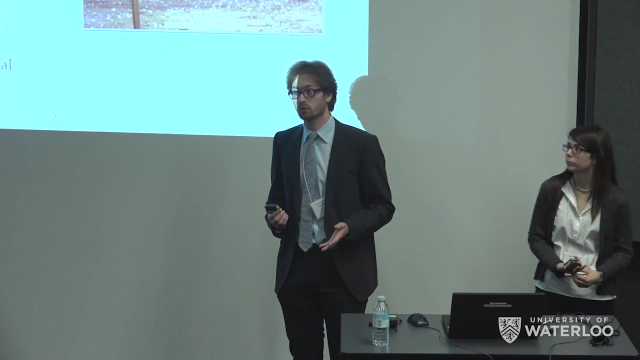 approaches and continues on, And as competition demand for sources of clean water increases, so will solutions for water pollution also increase in demand. Excessive heavy metal pollution in water is a problem often caused by industrial output or industrial runoff, and it poisons the water supply in many places. Some examples of this are for copper. 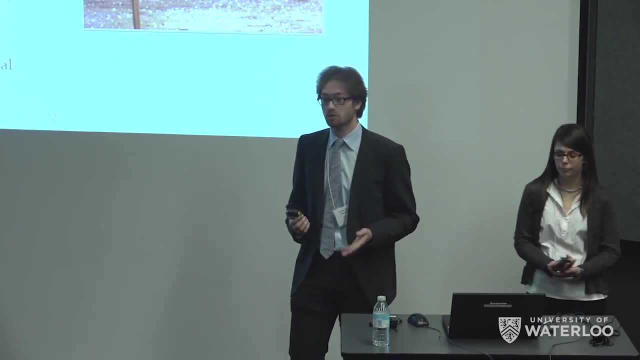 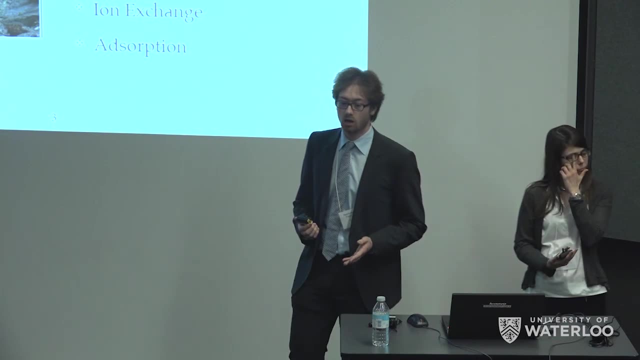 they can cause liver damage, lead can cause brain damage and mercury is just overall going to kill you. So the problem we're looking at is how do we extract these heavy metals from water. There are a few current solutions, such as reverse osmosis. 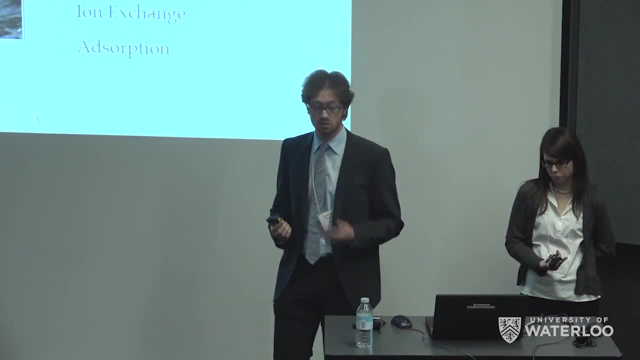 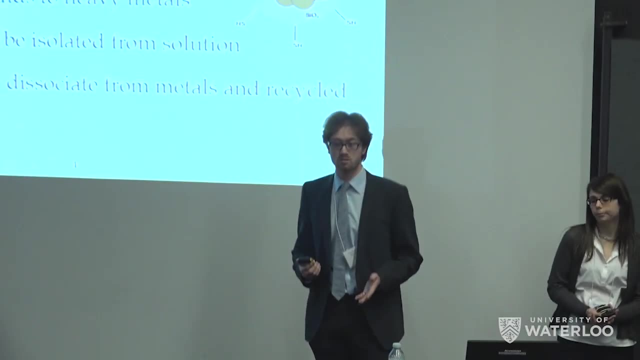 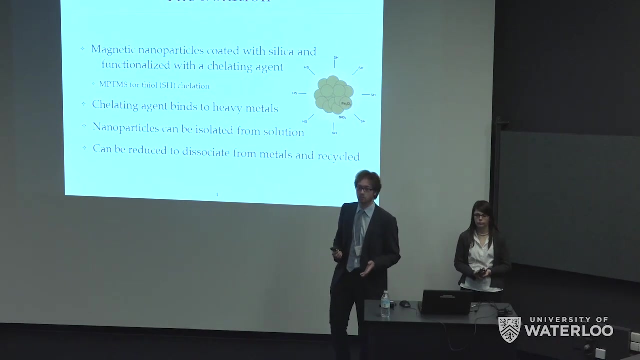 which is just inefficient: Ion exchange, which can be slow, and absorption as well. So our solution that we've proposed is that we're going to use magnetic nanoparticles that have been coated with silica and then functionalized with a chelating agent. This chelating agent that we chose is MPTMS, which is a TEOS molecule modified with a thiol group. 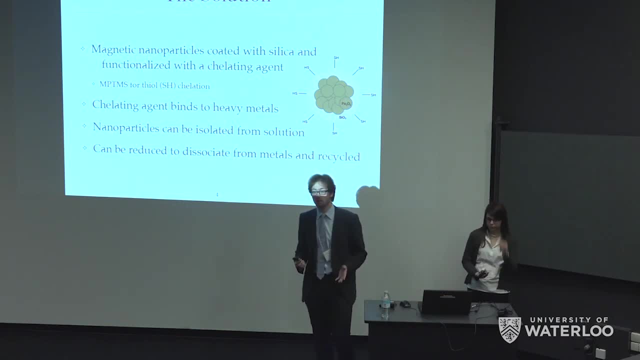 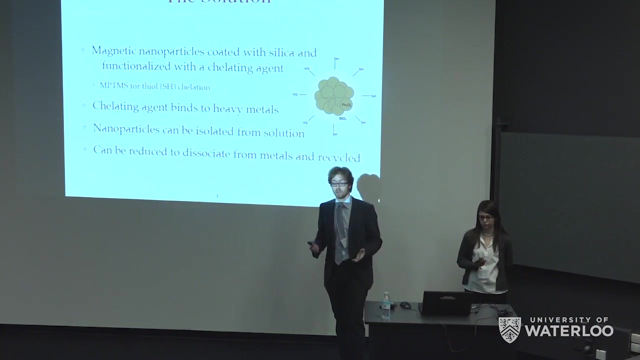 These chelating agents will form a chelating bond with heavy metals, removing them from the aqueous environment. What we'll then do is, because these particles are magnetic, we can use a strong magnetic to separate them from the water and therefore purifying the water of these heavy 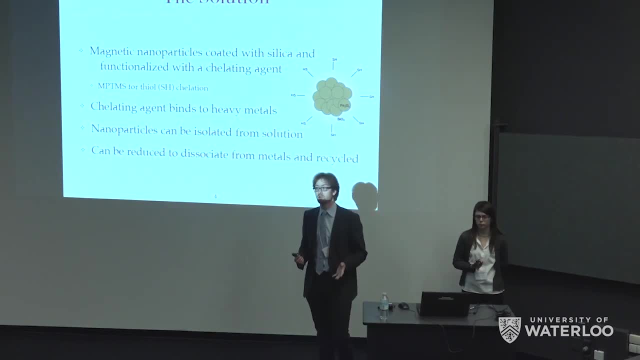 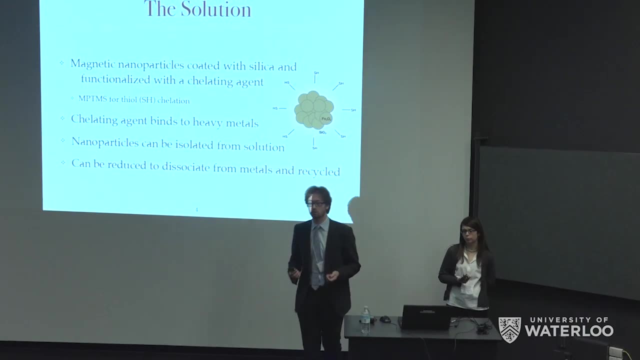 metals. Now, the neat thing about our nanoparticles is they are designed so that they can be recycled for additional use. With the addition of a reducing agent, the chelating bonds will break, and the chelating bonds will break and the chelating bonds will break. So we're going to 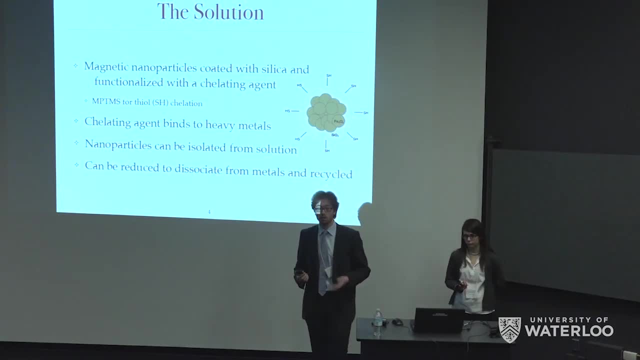 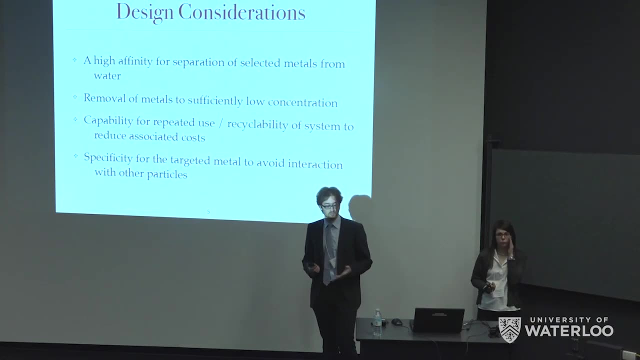 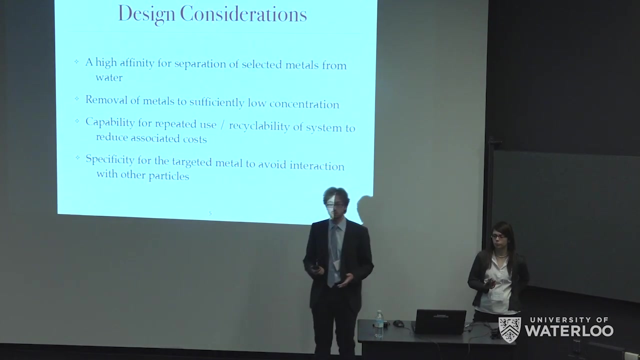 remove the chelating bonds and the heavy metals will dissociate from the nanoparticle, allowing it to be used for further usage. There are a few design considerations that have to be kept in mind. We require a high affinity for the nanoparticles for the selected metals. We want to remove the heavy metals to a sufficiently. 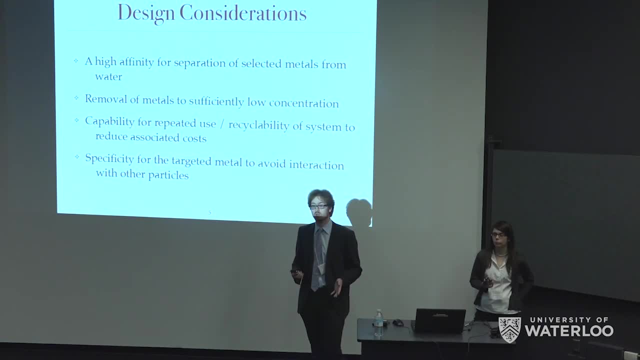 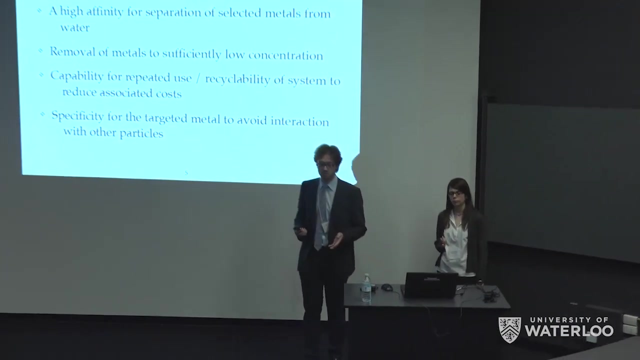 low concentration so that, ideally, they'll be within the safe drinking water limits. This is our goal at least. We want our nanoparticles to be capable of repeated usage, for recycling capability and to reduce it costs of the material. Finally, we'd like specificity for the target metal to avoid interactions. 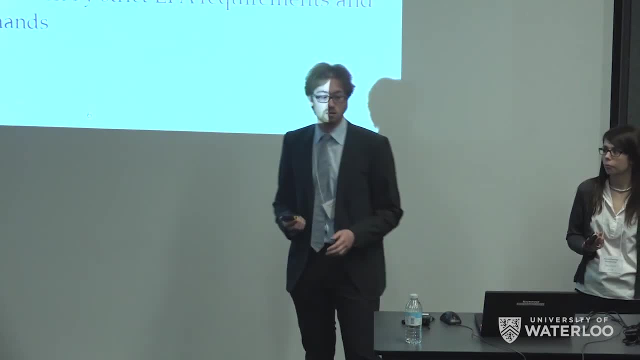 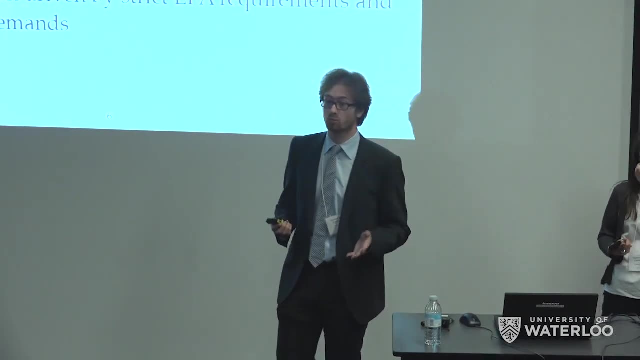 with other particles. The heavy metal removal market in the United States is 1.8 billion dollars. This is removal of heavy metals from wastewater, of course. The consumers for this are heavy industry and chemical plant in оч, PROFG mendels, and the United States is 1.8 billion dollars and this is for removal of heavy metals from waste water, of course. The consumers for this are heavy industry and the consumers of this are heavy industry, but it's not exactly really free of cost. it is, of course. It's kind of like viruses leaving można. The decommission collection now ends up suceders in the know, and if that doesn't work, we'll feel wrong. 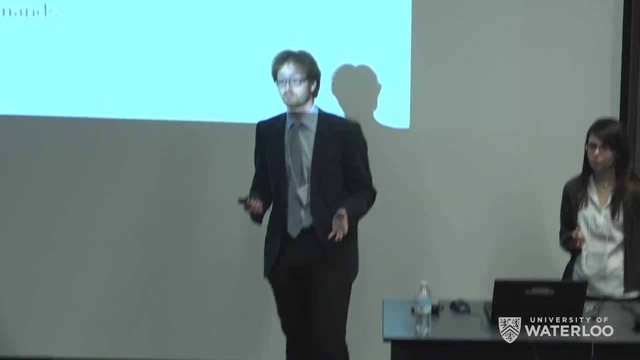 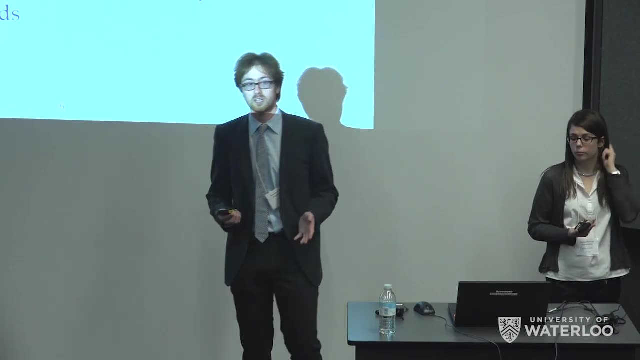 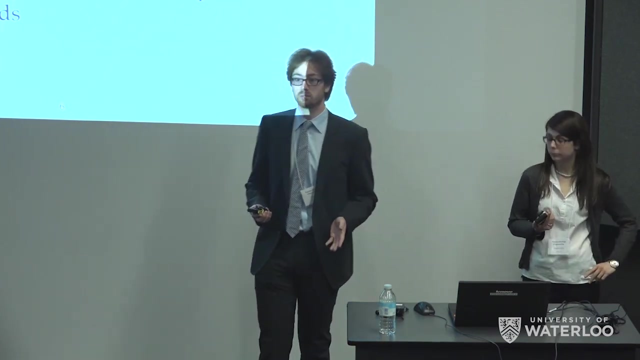 The consumers for this are heavy industries, water treatment plants and other government organizations. Industry growth is driven in part by new, more strict EPA regulations on certain ions in water, as well as consumer demands for more environmentally friendly companies. Megan will take over from here. 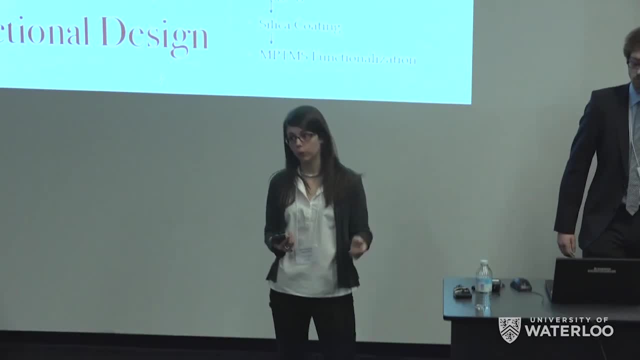 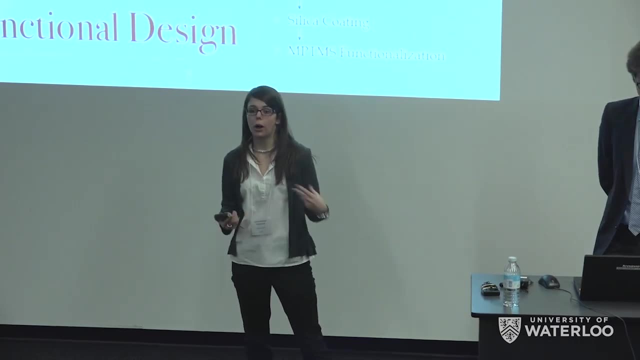 So, really quickly, we're going to go over the synthesis process of just how we're going to get these nanoparticles that are going to chelate with metals, as well as the functional design and how you can expect these to work on both the lab scale. 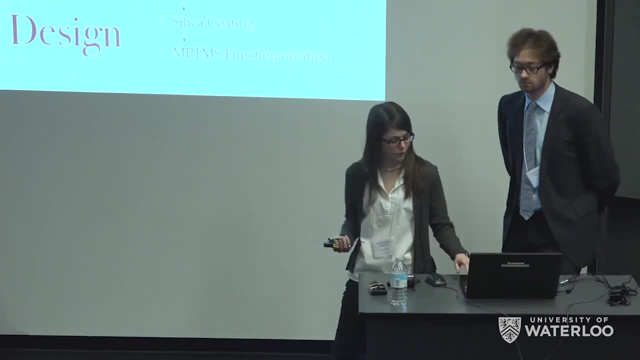 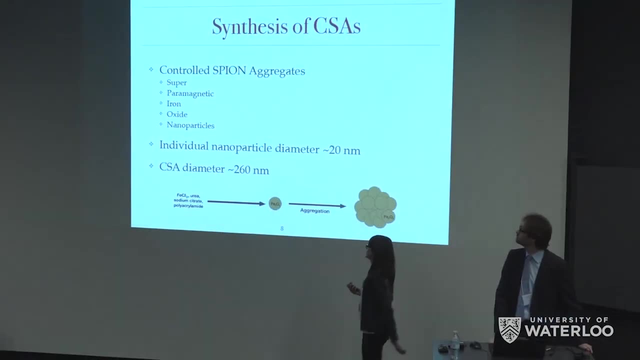 as well as the scale up onto prototype or industrial scale. So to start off, we first have to synthesize controlled spion aggregates. Spions are superparamagnetic iron oxide nanoparticles. So our starting point is right here. Based on TEM imaging, we were able to get size approximations. 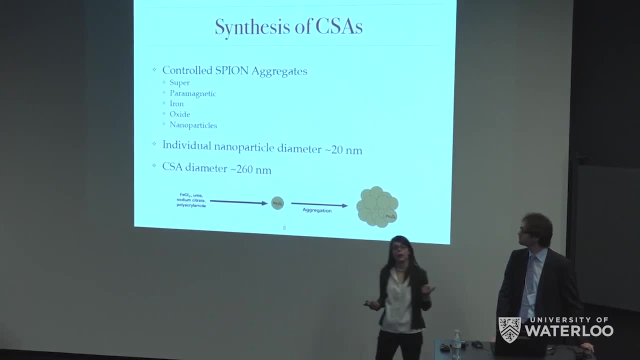 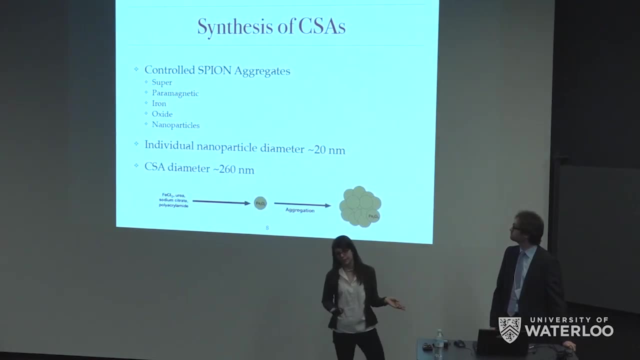 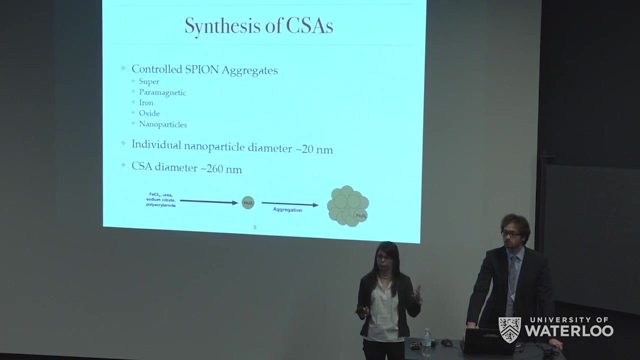 for our prototype. So the iron oxide nanoparticles start at about a 20 nanometer diameter And once they aggregate together, the CSAs have a diameter of closer to 260 nanometer. So this aggregation process gives us these nanoparticles which we can visibly and very fast. 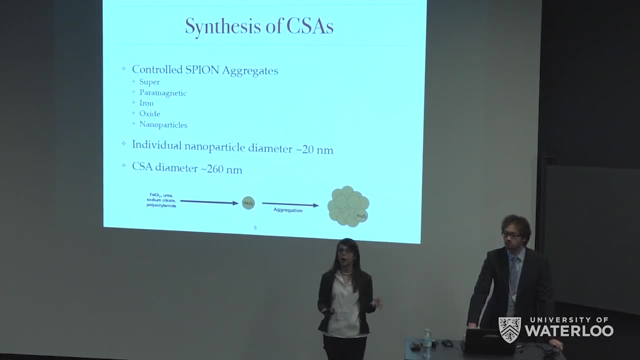 extract with a high-power magnet. We used a 1 Tesla magnet on our lab bench. The only thing is we can't do much higher for safety reasons, But there are more strong magnets on industrial scales which could make this even faster. Following this, we have to functionalize it. 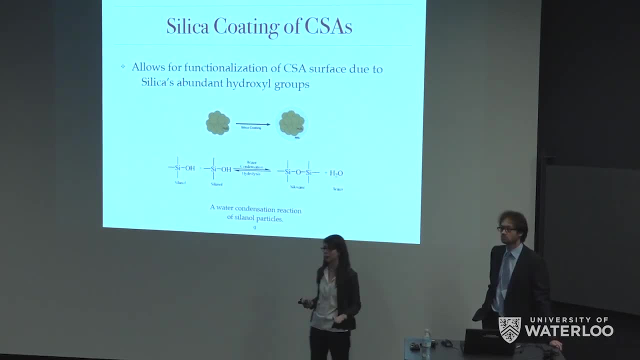 with silica, because the iron oxide themselves don't have any affinity for the metals, So we're going to have to synthesize it with silica, because the iron oxide themselves don't have any affinity for the metals, So we're going to have to synthesize it with silica. 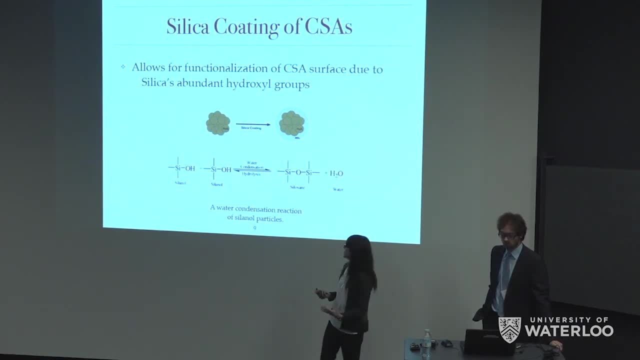 So, in order to functionalize it, we first use TEOS to coat the surface of the nanoparticles, And this silica coating can then be further functionalized with the ligand that's going to give us our properties. So, after the functionalization, these particles again. 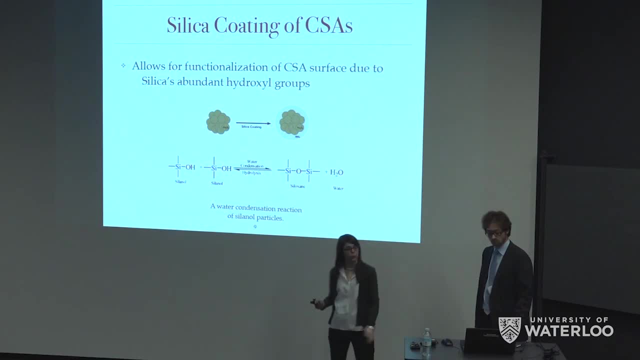 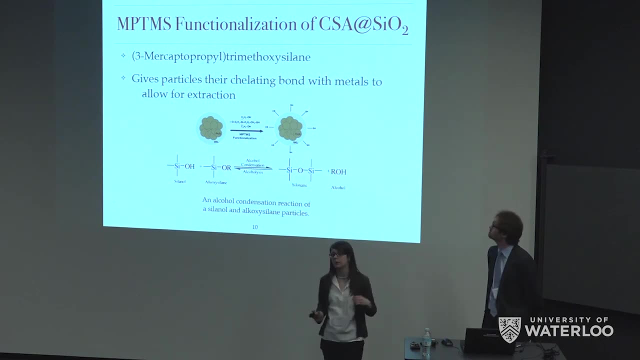 grow in size just due to the coating. And again, TEM imaging is going to give us the size approximation for that. The functionalization was with a molecule called MPTMS, which is quite a complicated molecule, But the thing of interest is that it. 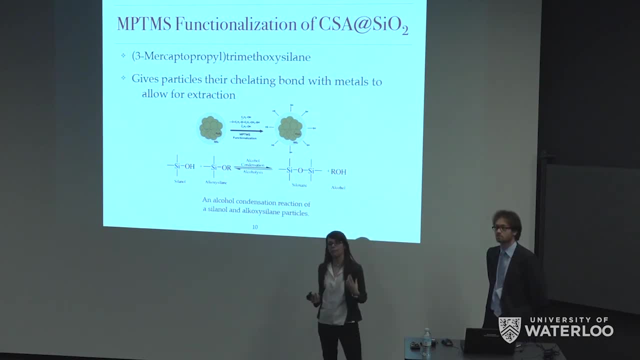 can be functionalized onto the silica surface and gives us these thiol groups which will form the chelating bonds with the metals of interest. So after this three-step process, we can confirm the synthesis after each step, which methods we will discuss in a moment. 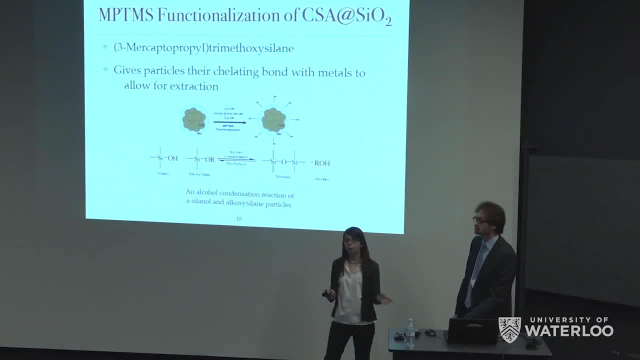 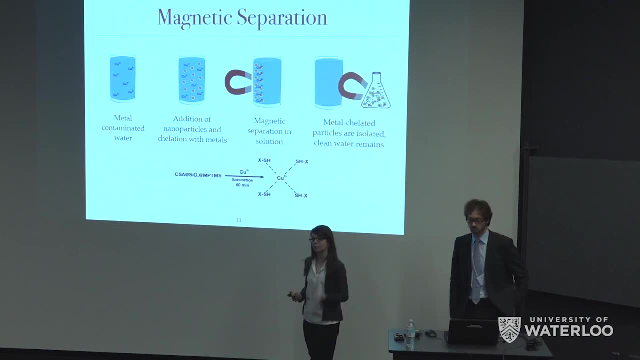 And these metal nanoparticles should be both magnetic as well as have the affinity for the metals that we wish to extract. So the process is relatively simple. You're going to start off with your metal contaminated water in some sort of fixed solution, so it is a batched process. 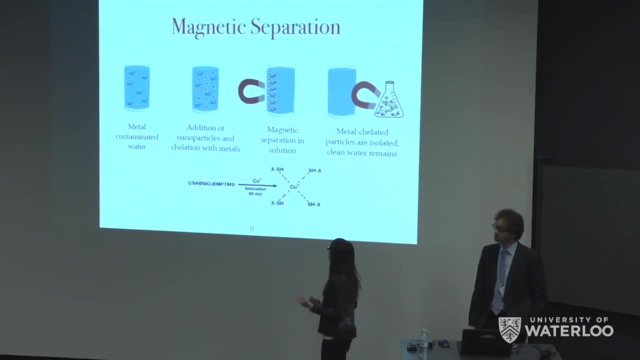 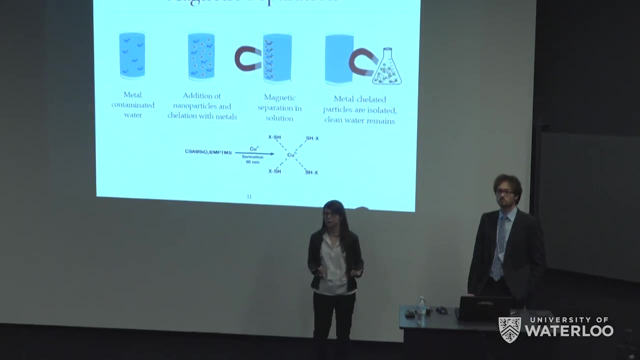 And you're going to determine an approximate concentration of your metals And, based on that, you're going to add a given amount of your nanoparticle to the solution that will be able to remove approximately all of the metals. Once you're in there, you're going. 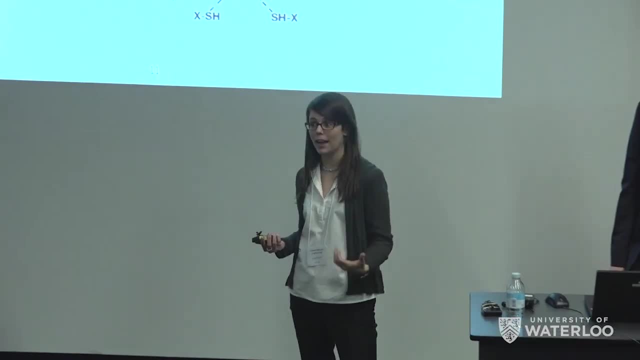 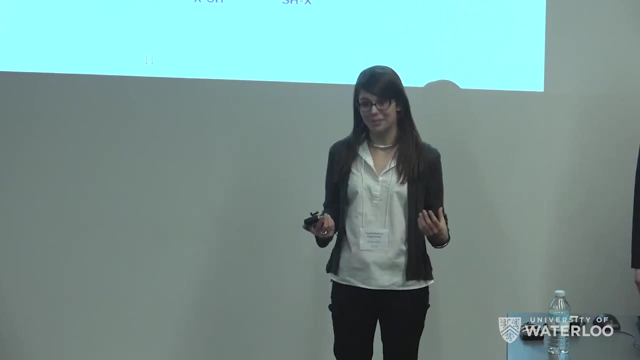 to want to let it to mix to allow for the chelating bond to happen. In our lab test we use probes on occasion for 60 minutes, which is somewhat overkill. That is very thorough. So we do not think that there is any limitation, just due 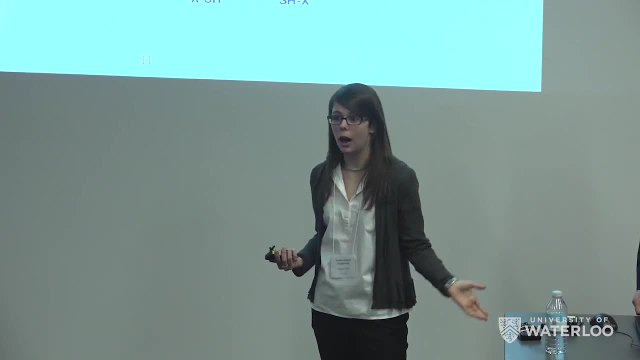 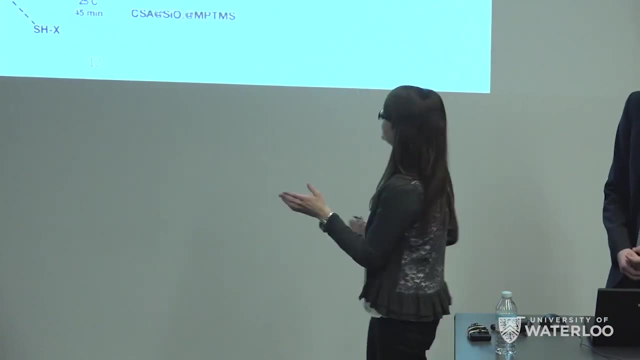 to our mixing process. This could likely be scaled down to simple just stirring for a shorter amount of time, because this isn't a very time-limited process. Following that, you use a magnet to separate the particles to the side, which should have all of the heavy metal. 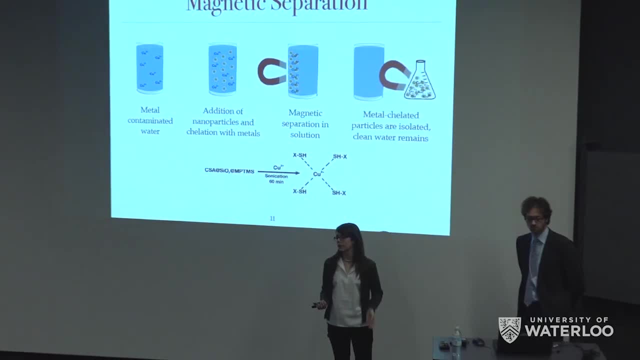 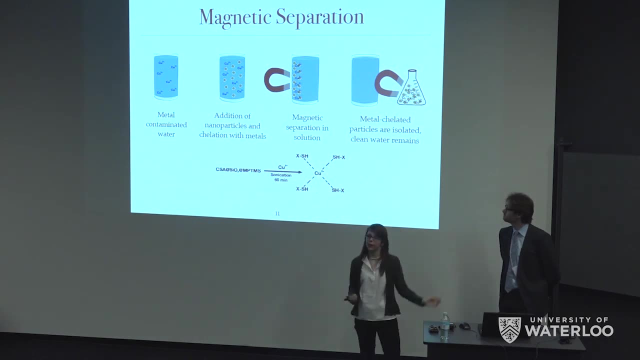 in solution with them. The solution can then be decanted off or the magnet themselves just separate. We decanted it off quite easily, And so the metal chelated particles can be isolated from the solution. Following that, the recycling process is even simpler. 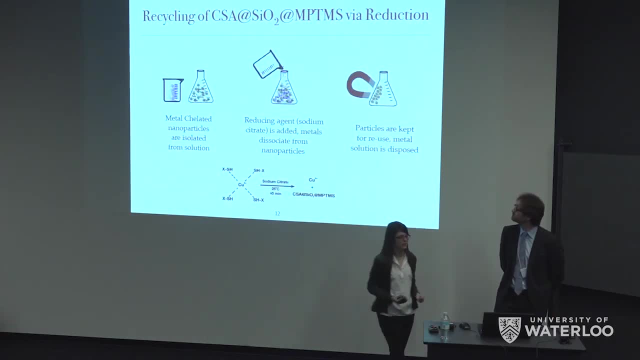 Sure, Our nice pink dust here is used to represent any form of reducing agent. We use sodium citrate and simply you add it to your solution. you stir it for a sufficient amount of time. We did it at room temperature. Potentially you could increase the temperature to get more reduction. 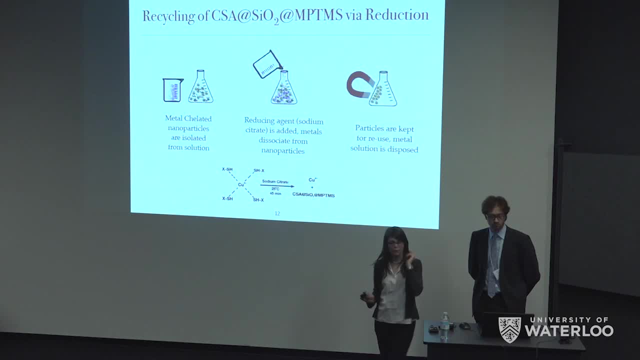 but our testing was completely fine. like this And following this once again, you'll use magnetic separation and the solution that comes off should be the metal-contaminated solution and the particles that you pull off should not have any metals with them. 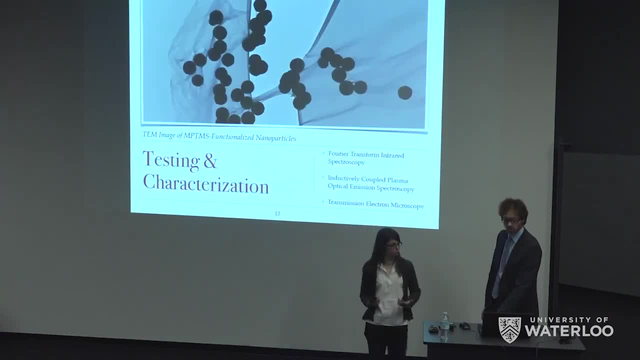 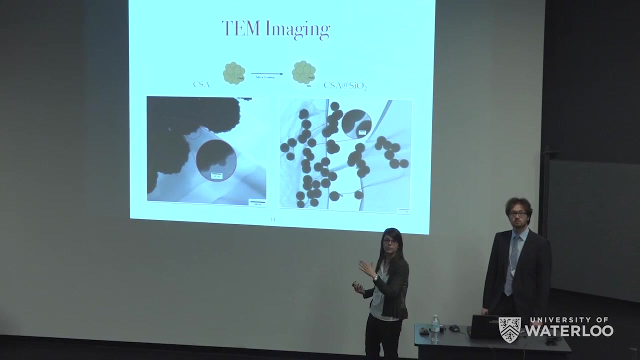 So once again you can just reuse them again in the separation. So to actually characterize and test our particles we used a variety of techniques, first to confirm our synthesis and then to take a look at the efficacy of the metal separation. So to start we did TEM engine to first confirm both the synthesis of the CSAs. 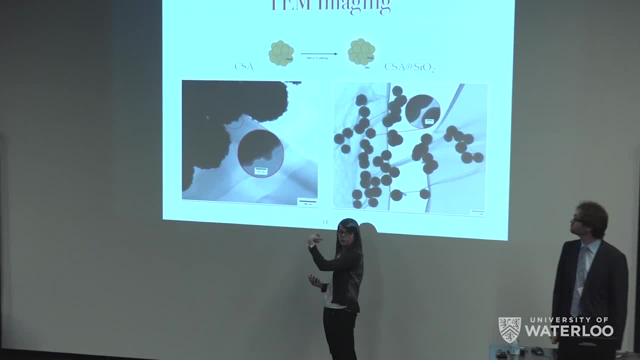 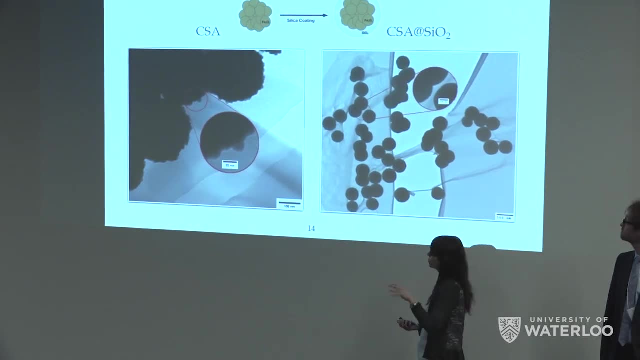 the aggregates, which you can see visibly by the smaller nanoparticles, as well as the aggregation with the diameters, again, of what we mentioned, of 20 nanometers for the individual particles and then closer to 260 nanometers for the larger aggregates. 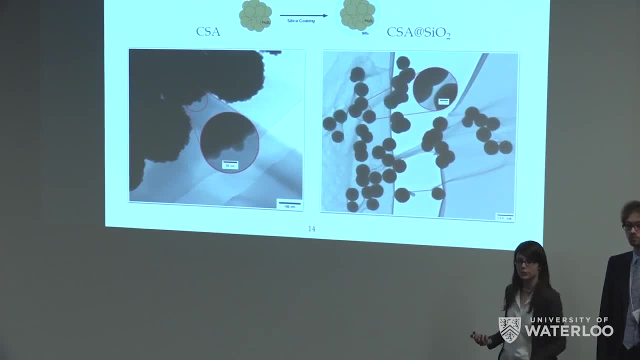 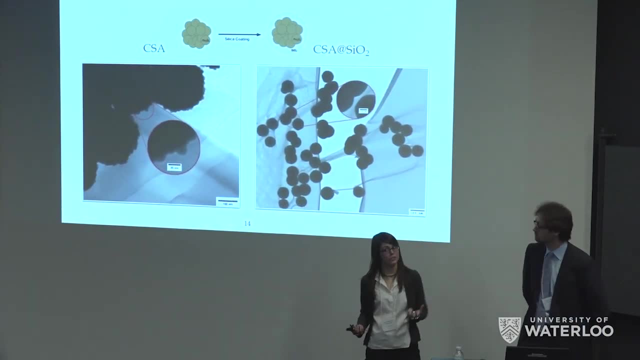 And then after the coating with silica, which we see a much smoother surface of silica surface on these aggregates, as well as a larger diameter, closer to 470 nanometers. So these are actually quite large nanoparticles. So this is the one that we are then going to functionalize with MPTMS. 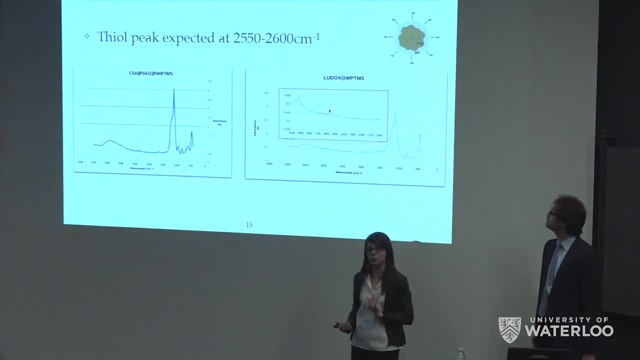 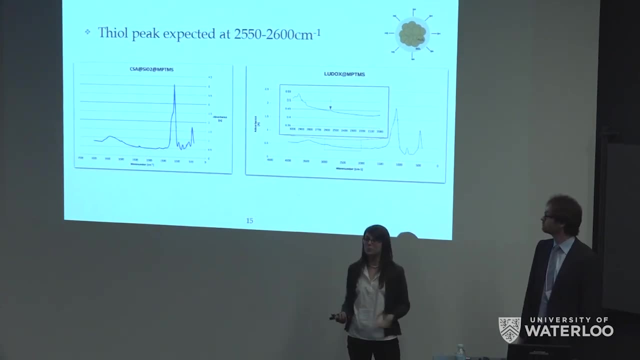 And the MPTMS functionalizing was a little bit more difficult to actually confirm. We attempted to use FTIR to begin to try and look for the file peak of interest which we were Most caring about in order to get these chelating bonds. 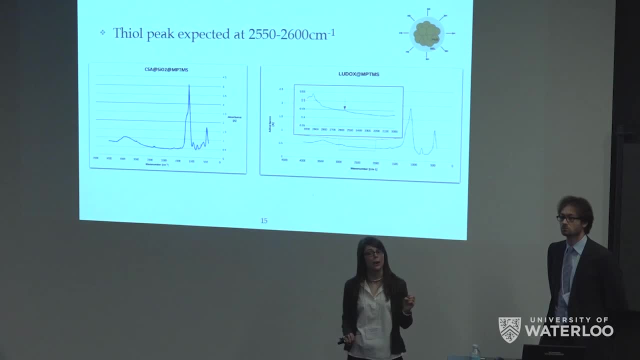 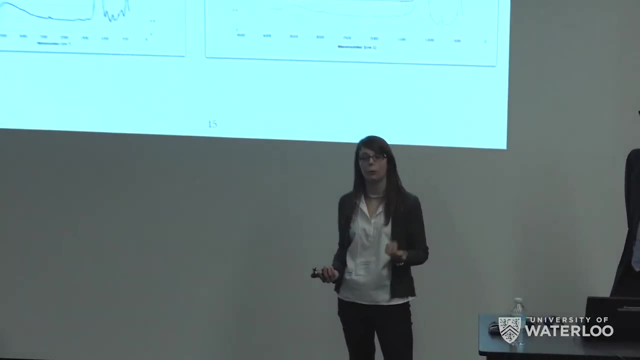 But just due to the size of the nanoparticles, the file peak was actually quite, quite small. on our nanoparticles themselves, If you can imagine the 470 nanometer diameter, the majority of the mass is going to be both the iron oxide as well as the silica coating. 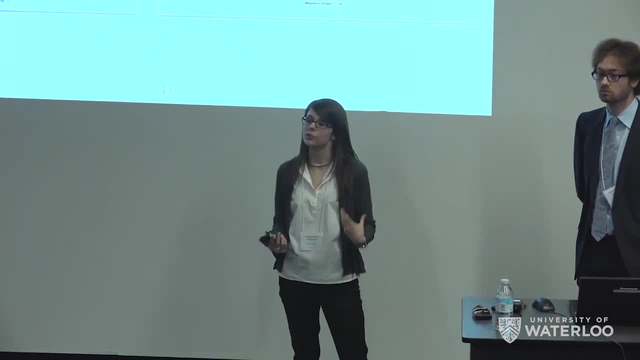 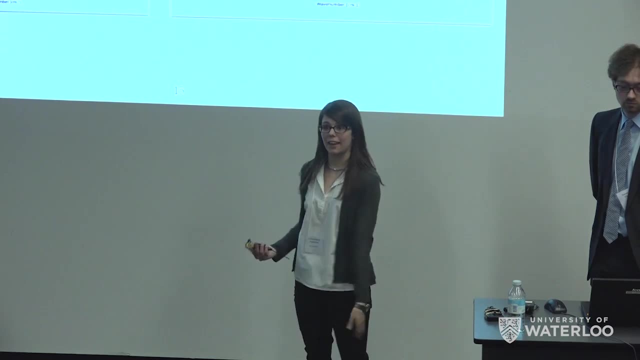 So what we actually thought about is if we could just prove that the functionalization mechanism works on silica and we can see file peaks on that functionalization, we could then say: this functionalization is going to be a little bit more efficient. So we could then say: this functionalization is going to be a little bit more efficient. 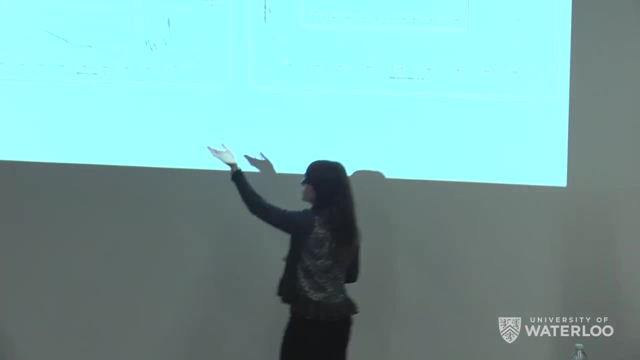 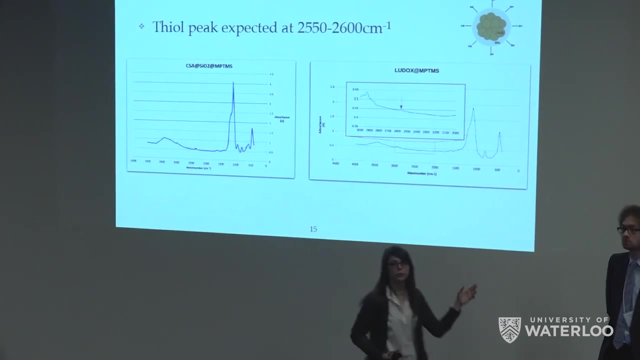 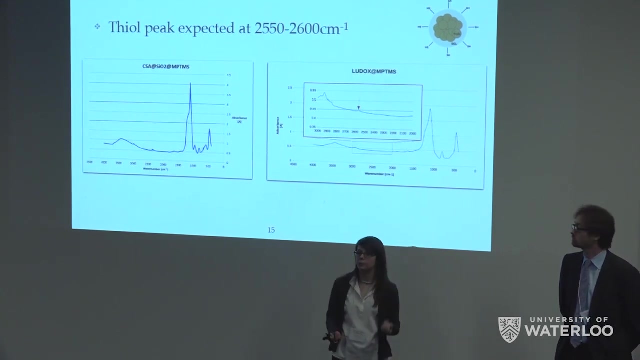 So we could then say: this functionalization yields the file peaks that we want. So after FTI results of our nanoparticles with the silica coating, we're unable to find a file peak, Our workaround is that we use LUDOX particles, And LUDOX are approximately 26 nanometers in diameter, but just of silica dioxide. 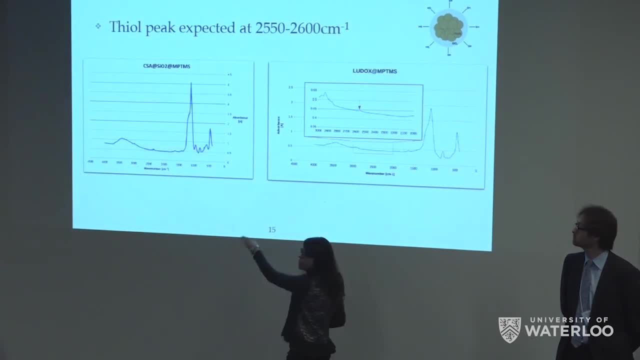 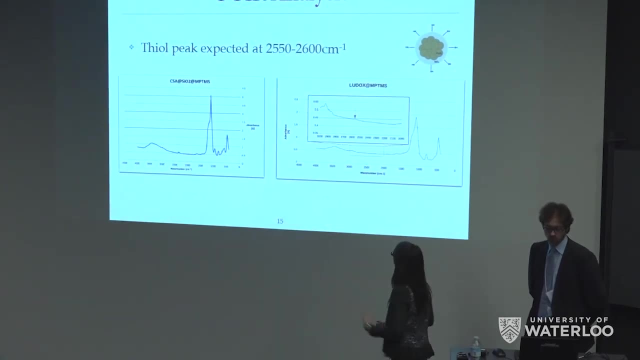 So the functionalization is identical for both systems, aside from this being larger and this being smaller, And, as a result, we actually were able to find the file peak where we expected between 22,515 and 260 nanometers. Again, it was quite small, so it's very understandable why we would lose it. 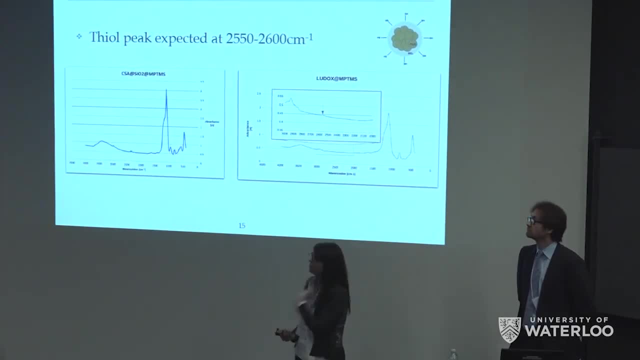 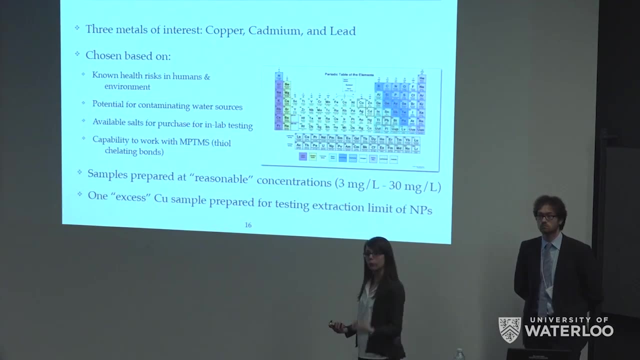 in the larger nanoparticle. But after this confirmation we were able to go on into the actual testing process. So our testing plan was going to focus on three metals: copper, cadmium and lead. These were chosen because they were known health concerns for humans. 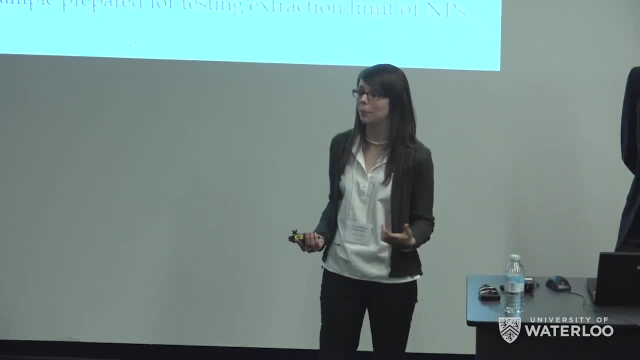 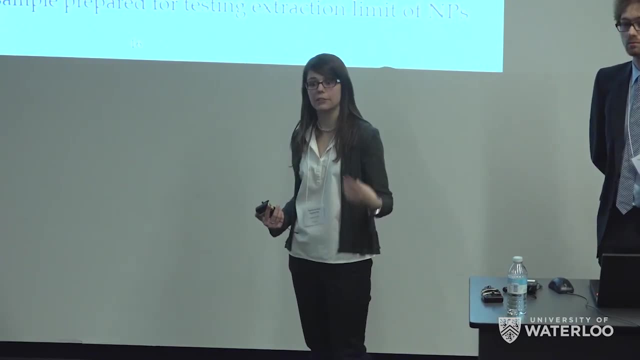 They are known to be actually found in water, contaminant commonly, be it from industrial waste or other runoff sources. as well as the capability of the silica coating, They are known to have the capability to work with MPTMS to form chelating bonds. 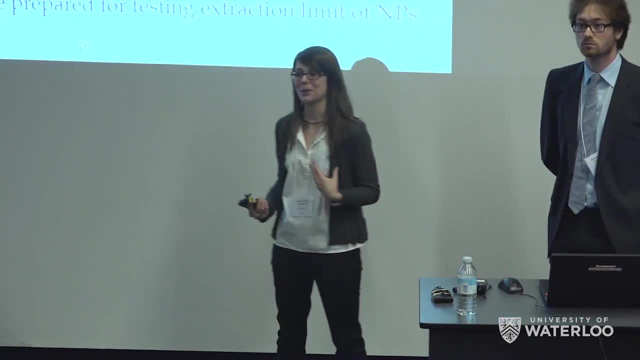 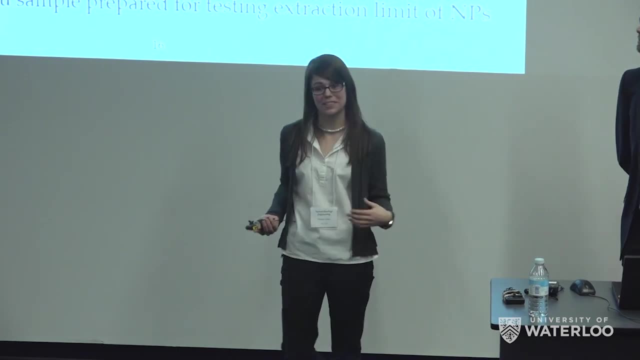 as well as just available salts for us to work in the lab and to purchase. We were interested in testing mercury as well, just due to the prominence of its health effects, as well as relevancy in terms of the pollution in, for example, grassy narrows. 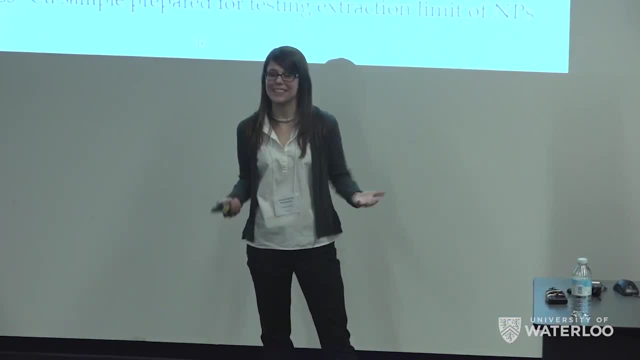 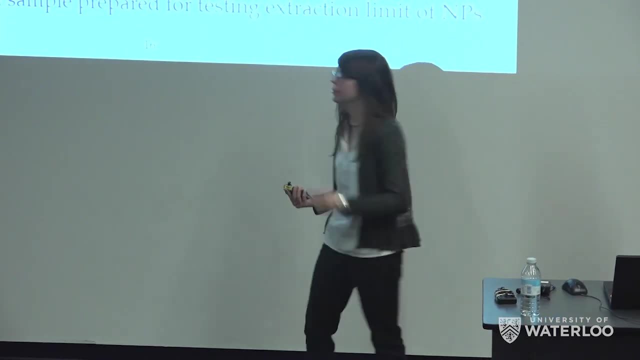 There's a large mercury concentration to be removed. But health and safety? we can't work with mercury in the lab, But the in theory, the same sort of chelating principles could be applied to other metals as well, so we just focused on these three. 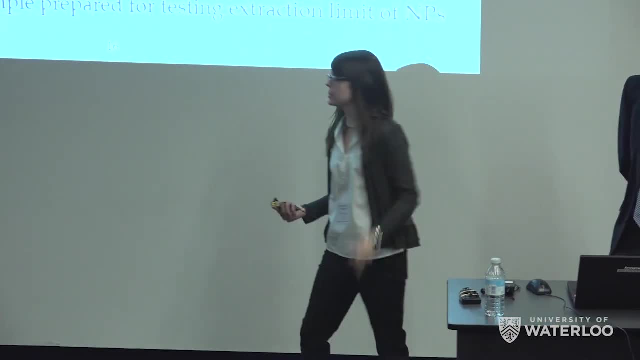 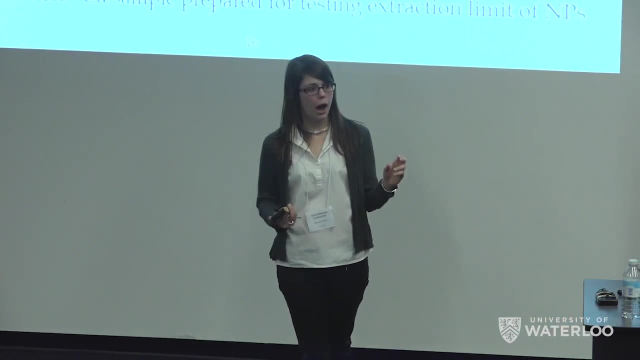 We then prepared samples- two types of samples. The first type were prepared with the metal salts at a reasonable concentration, So we're talking about 3 to 30 ppm in solution, And then we were going to test them with our nanoparticles to see before. 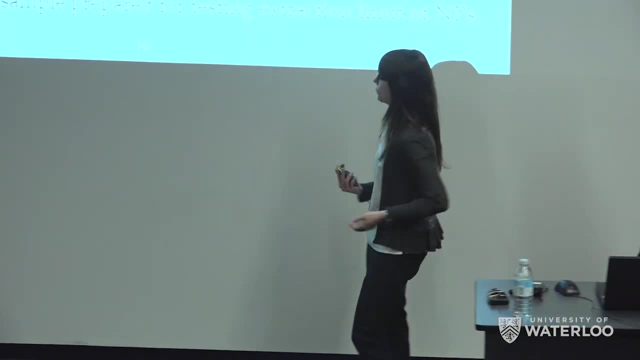 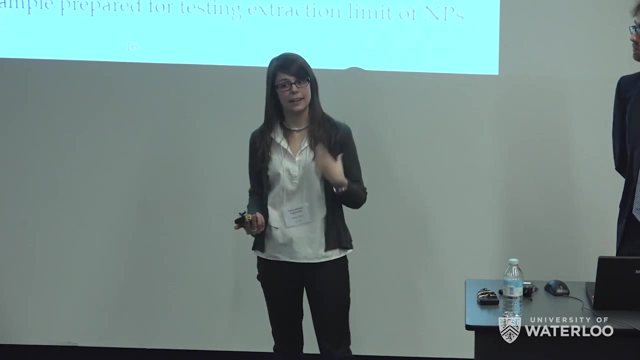 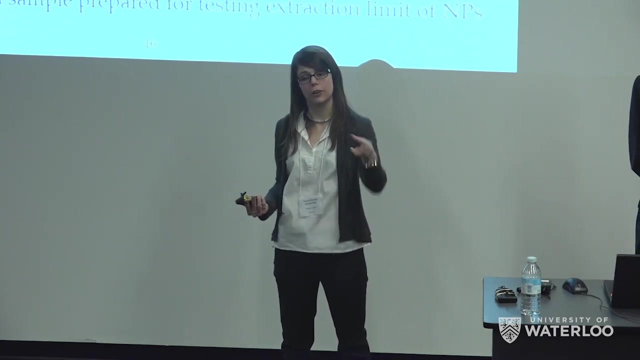 and after just how much metal we removed. A second sample that we used was actually only copper, but there was an excess of copper in the solution And what we did is we tested it in the exact same procedure with our nanoparticles, But whenever we tested the extraction, we didn't test the extraction of the copper. 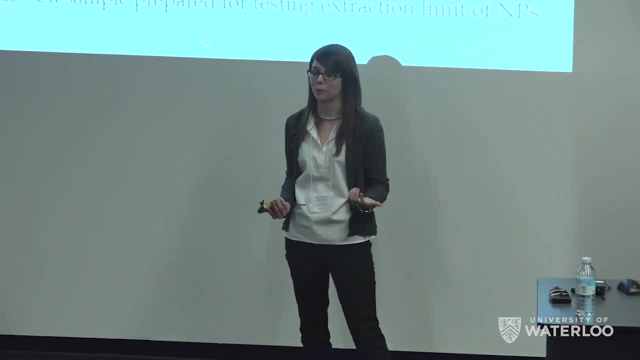 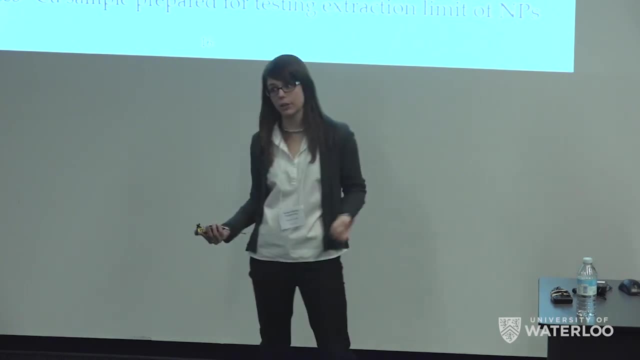 because there would still be an excess. Of course, our small amount of nanoparticles couldn't remove it, But we tested afterwards, when we recycled the particles, just how much copper came off after the reduction process. So we looked at the elutin after reduction. 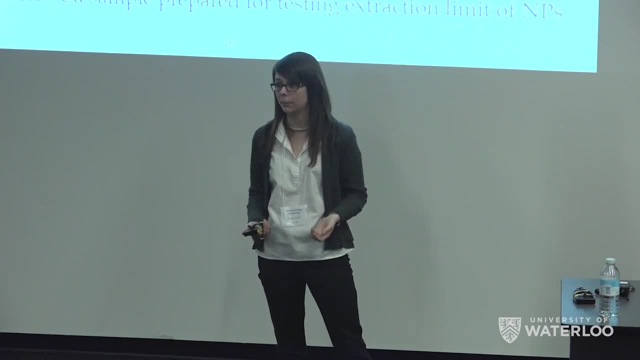 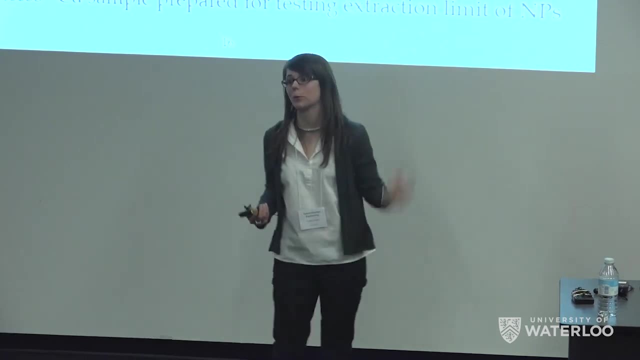 And in theory that should be the maximum capability for our nanoparticles in order how much copper they could capture. So by putting it in a excess solution We can kind of test that upper threshold and, just in an ideal situation, how much copper you could get off. 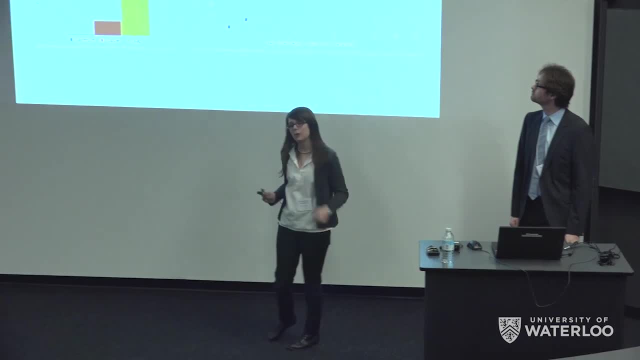 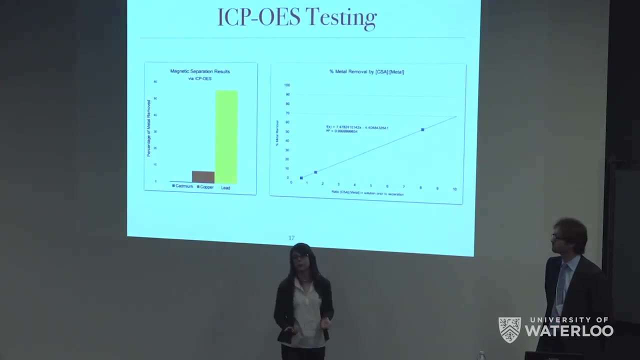 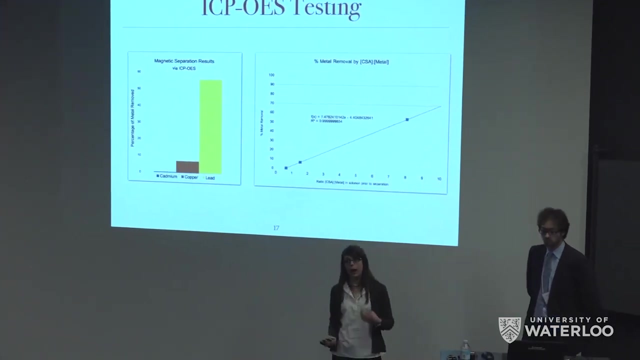 So our testing results for ICP were mixed. We had a very good result in terms of our lead yield- It was over 55% of the concentration was removed- But for both cadmium and copper we actually had weaker results, And so we're going to talk a little bit about how we think both of the 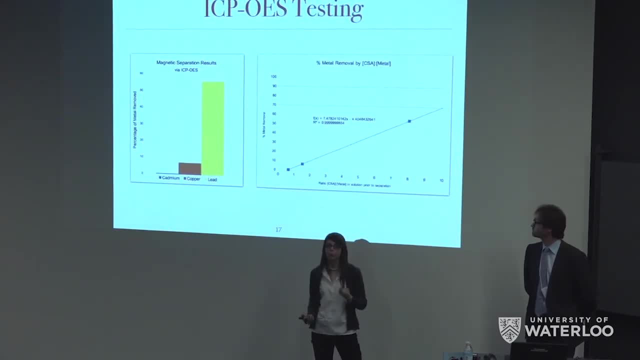 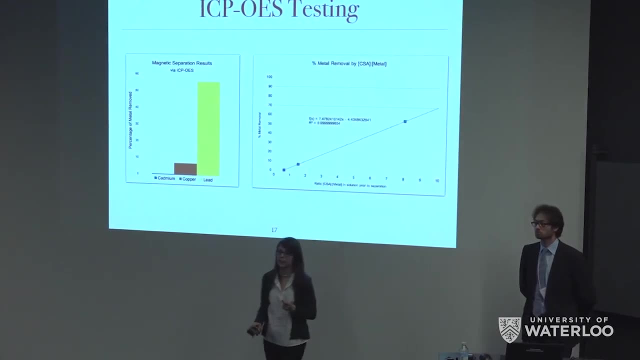 how to explain these results. But a lot of it, we think, has to do both with optimization of our particles as well as with our testing technique, Because one thing we also noted is, just when looking across our different samples, there was a direct trend in how much nanoparticle we use per concentration of metal. 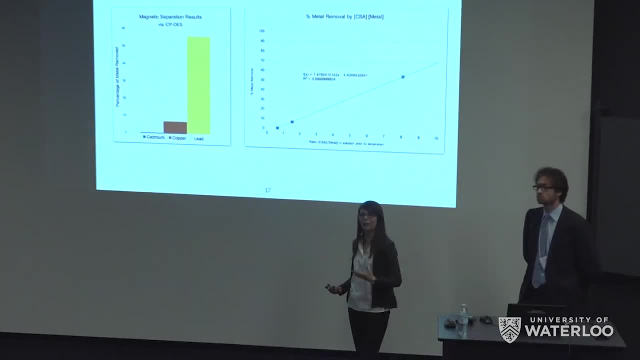 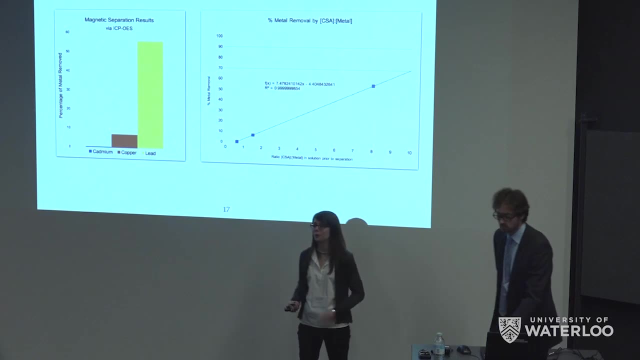 And it was very simply put. we were not putting enough of our nanoparticle into the solution to get rid of the amount of contaminant in there, So we simply needed to increase our dosage in order to remove it, And with time constraints we weren't able to do more testing. 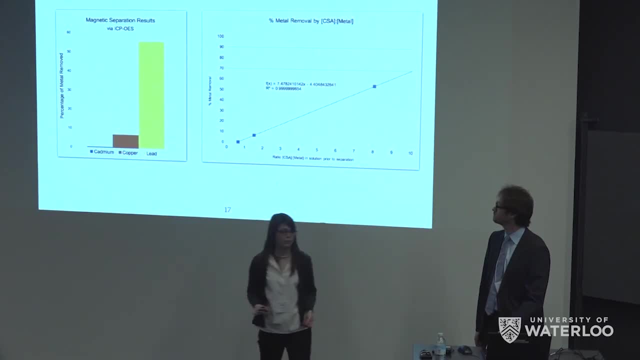 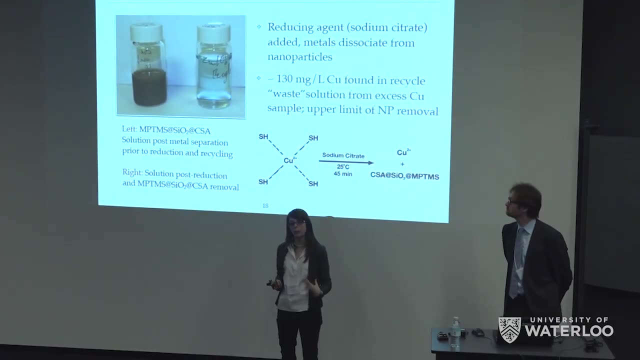 But the results are promising, so long as we can optimize our actual techniques. This is further proven when we take a look at the recycling of the product, Because whenever we took a look at the concentrations of the copper, that was reduced off of the nanoparticles post recycling of that high concentration copper. 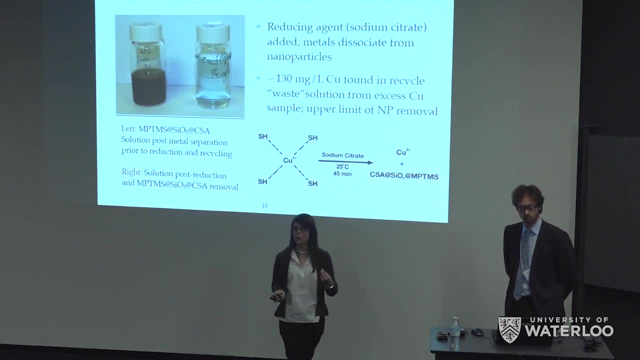 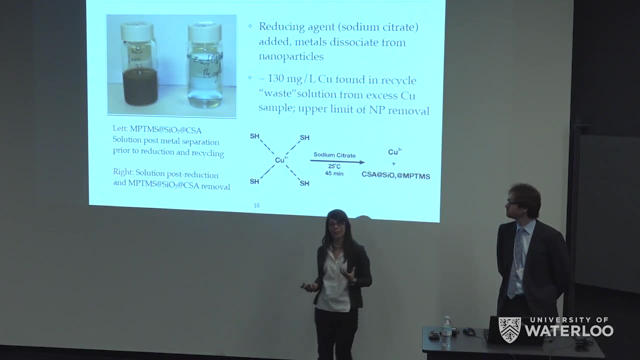 we were capable of seeing a very noticeable blue hue in the recycled elutin, which actually had a concentration of about 130 milligrams per liter, which is quite large. So the upper limit of our particles is actually much higher than the results that we were getting based on our testing. 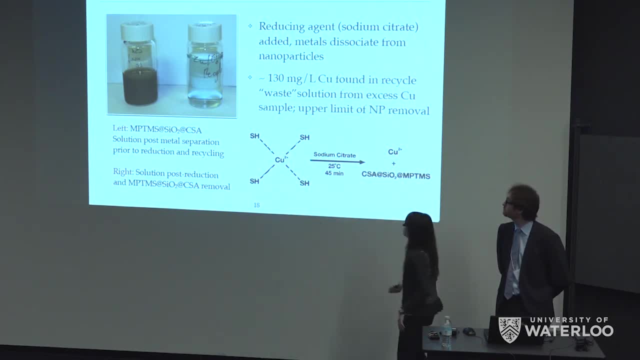 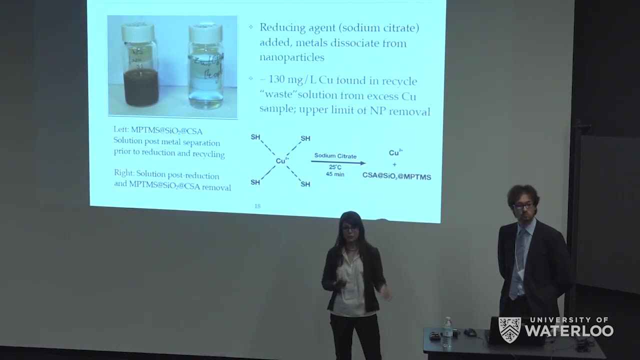 We just have an increase, So we can optimize the parameters. And again, once we tested these recycled products in a similar manner to the previous concentrations, we yielded similar results, which were again running at the suboptimal concentration of our nanoparticles to the metal contaminant. 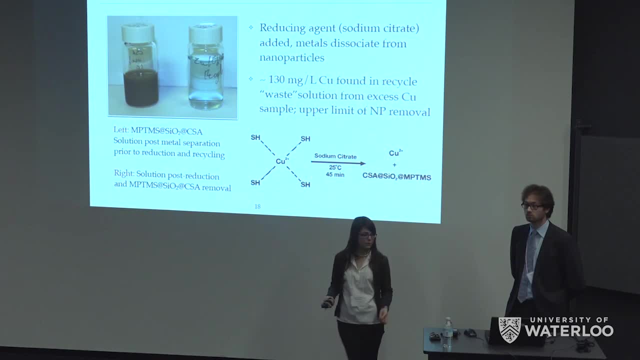 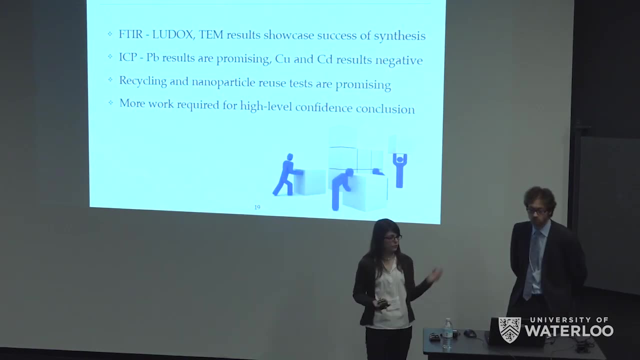 So the recycling process is showing promise, in that they have yield similar results as well as are showcasing the upper limit of potential of our product. So this is pretty much the summary: That we confirm the synthesis via FTIR, as well as TEM, of our product. 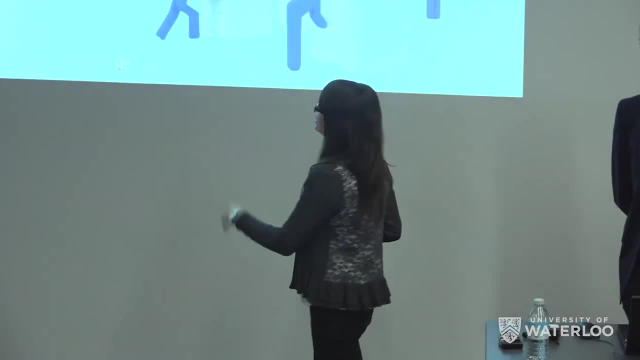 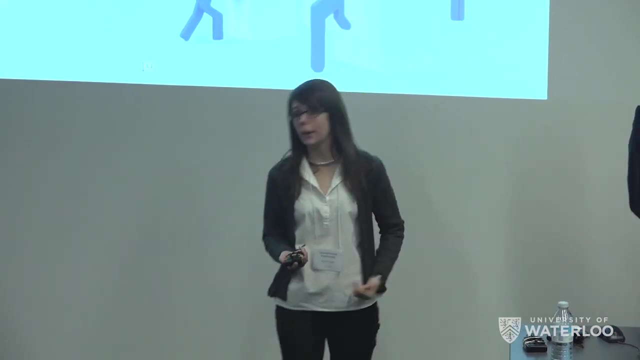 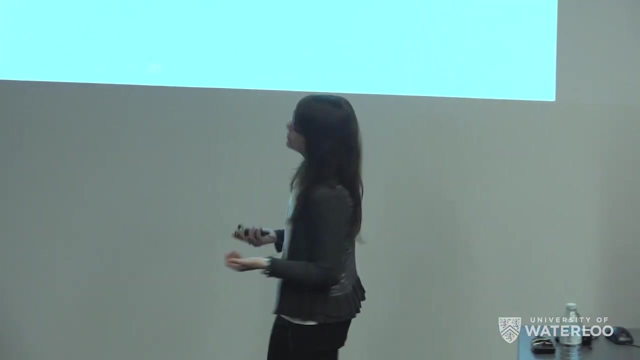 up until the MPTMS functionalization And via ICP we could test that we had some mixed results from the lead, cadmium and copper, but the recycling results are quite promising as to optimization of our product. So what can we optimize? 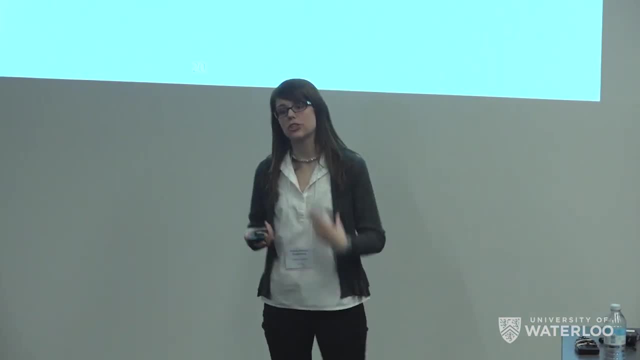 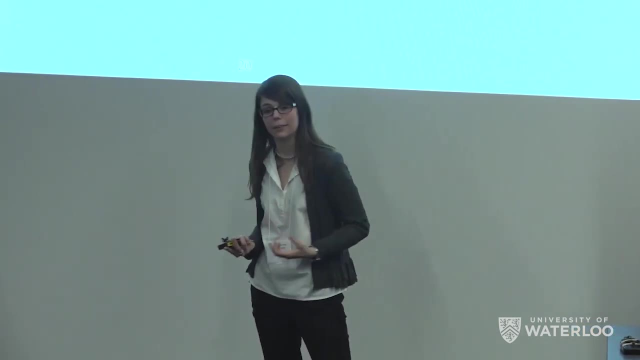 Just as we mentioned before, we're going to have to look at optimizing just how much material we are going to need per cadmium. So if you have the approximate idea of how much metal contaminant is in solution, how much nanoparticle you're going to need. 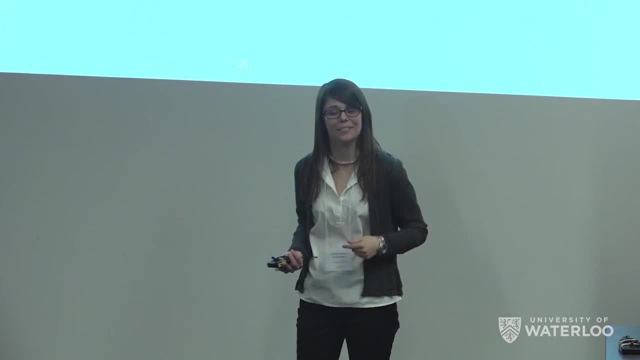 We want to optimize it so you don't have to add an excess, because that will be cost inefficient, but also want to have it so that you're getting a safe level. We could also look more into optimizing the extraction time. how much time we spent sonicating. 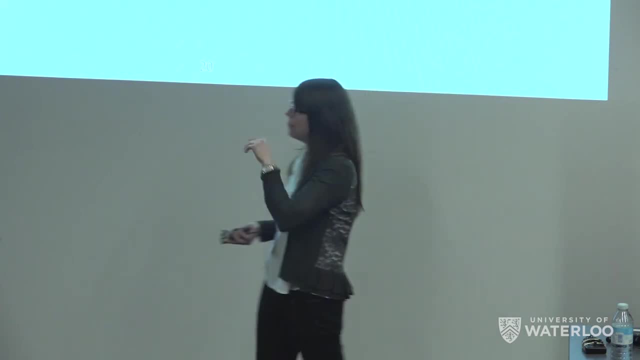 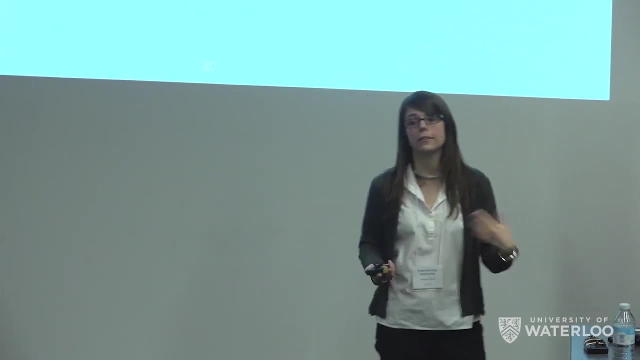 how much time we spent on the magnet, but that's more small details. But a very interesting idea that we had was looking at our synthesis technique of coating the silica layer on the nanoparticle. So we're going to have to optimize that. So if you have the approximate idea of how much metal contaminant is in solution, 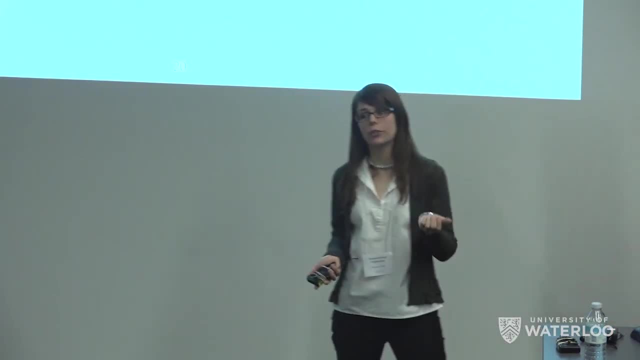 how much nanoparticle you're going to need. So if you have the approximate idea of how much nanoparticle you're going to need, Because, as you remember, TM images show that those were almost 500 nanometers in diameter. Those are quite large particles. 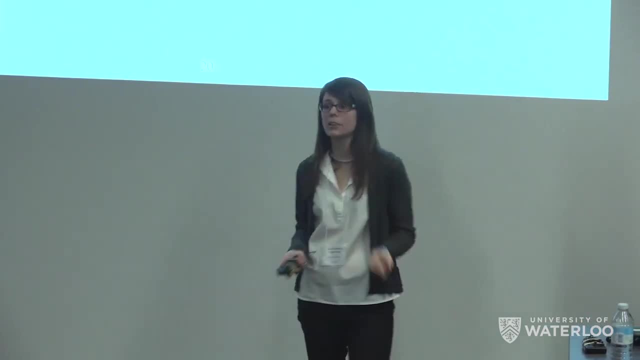 And while the coating of the silica is important in order to have the MPTMS, we think that by reducing the size of that coating, by making smaller nanoparticles, we will in turn have a higher surface area, which can make more file groups available. 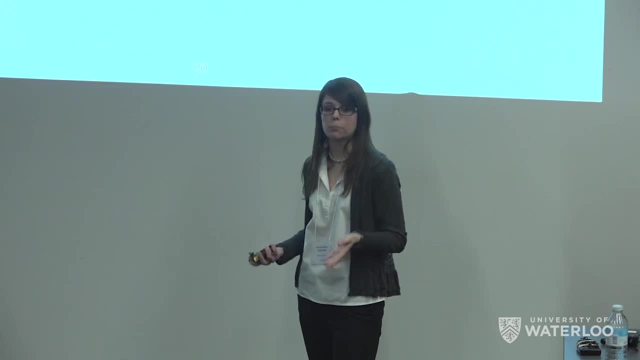 for chelating, which will once again make the particles more efficient per gram, And so, by reducing the size and surface area, the particles will essentially be more efficient, and you won't even have to add any more nanoparticles, And so, by reducing the size and surface area, the particles will essentially make the particles more efficient. 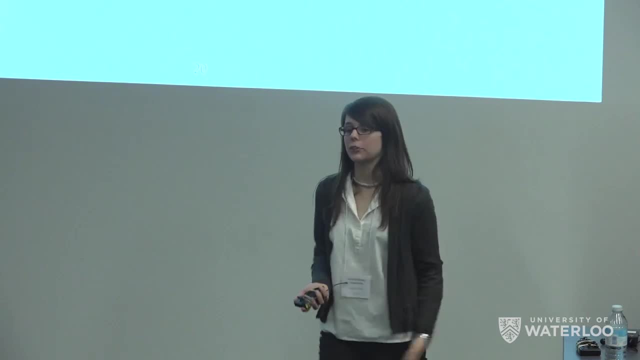 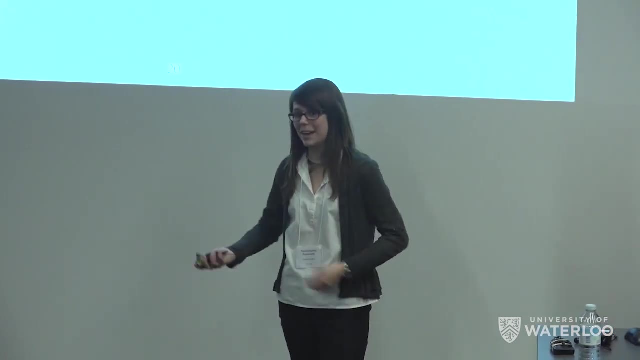 and you won't even have to add as much in order to remove the metals. And finally, just looking at the recycling process, similar to the other one: optimizing just how much metal you remove so that you're not introducing any more contaminants when you reuse the particles, as well as optimizing the yield of the recycling. 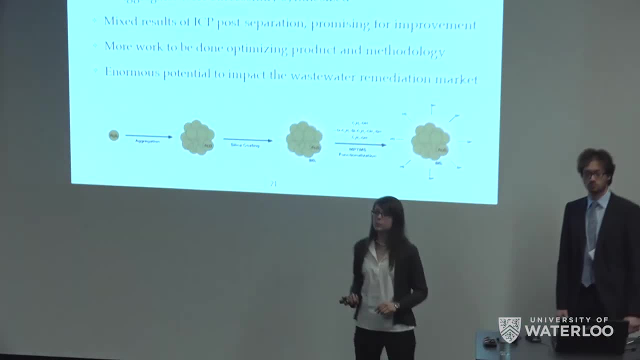 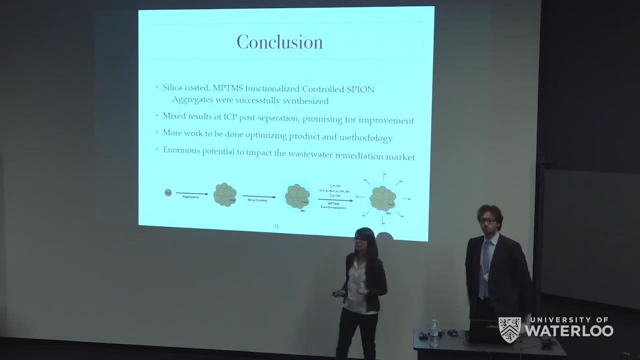 So, in conclusion, we have successfully synthesized controlled spion aggregates coated in silicon dioxide and functionalized with MTMS. These are going to be used for removal of heavy metals in solution And our IC figures are going to be used for the removal of heavy metals in solution. 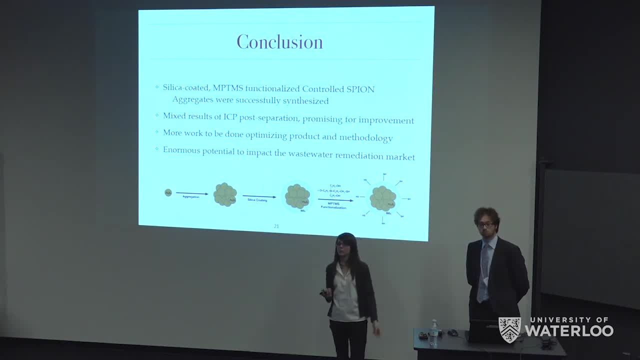 And our IC figures are going to be used for the removal of heavy metals in solution. We don't know if the results were mixed, but based upon these ICP results, as well as the results of the recycling of the particles, we see a lot of promise. 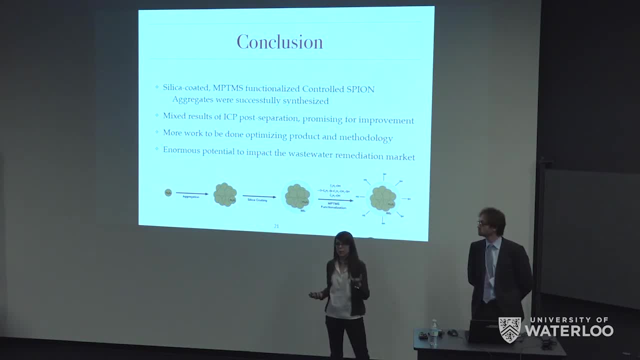 and just optimizing our particles, both in their size as well as their actual method of procedure, in order to break into the heavy wastewater market, And that's all for now. We'll be able to take any questions you have. Thank you very much. 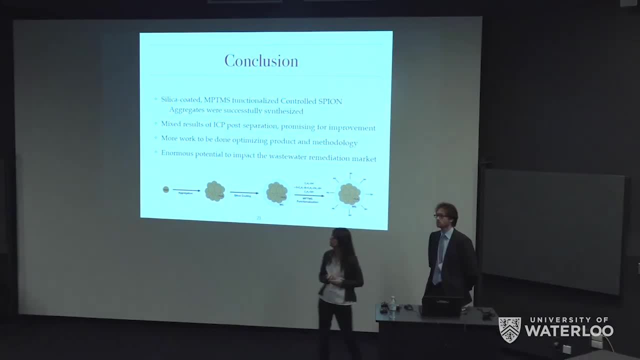 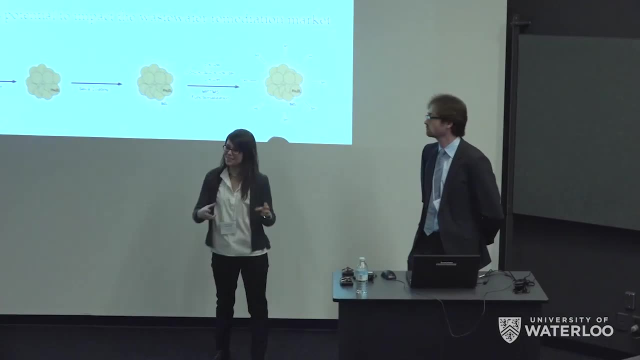 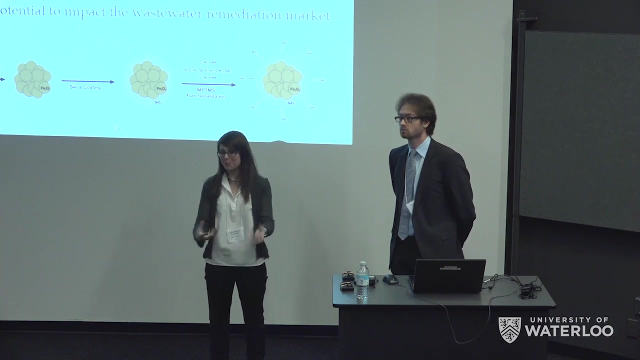 so, yes, we did do. our ICP testing was quite limited at the end of the term, but we were able to do one recycling test, again with the copper, but unfortunately, as we saw, like our copper results weren't great, but they were. it was comparable results in terms of. so we add a in order to 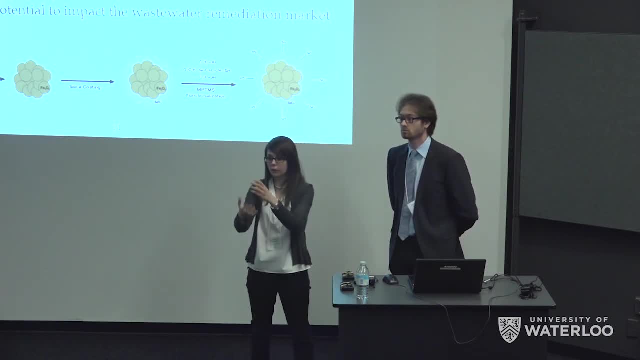 recycle it, we basically add the reducing agent, and when the reducing agent is going to dissociate the metals and so the metals will be in solution. so when you pull the magnetic particles out, the magnetic particles have no more metal on them and the solution will remain with the concentrated amount of the cost is somewhere in the range of a few hundred dollars per kilogram of product. this, the final number, will depend on the if we choose to make modifications to the nanoparticle itself. there's various ratios and the chemicals involved, but it's somewhere within that range. we have not done that. the one the one thing is is that, though 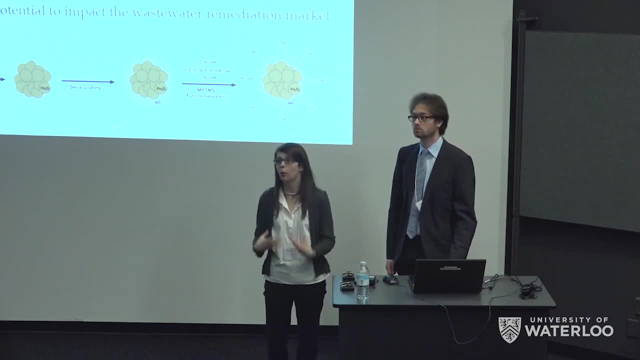 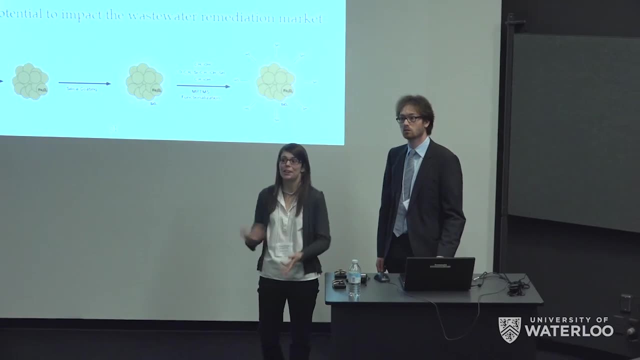 the particles are very easily dispensable in water. it's not like they're an emulsion or anything that you need that sort of sonication. even just like ten minutes of stirring should be efficient, sufficient. it's just the matter of us wanting to remove that as a parameter to consider. we had limited time to perform, to do. 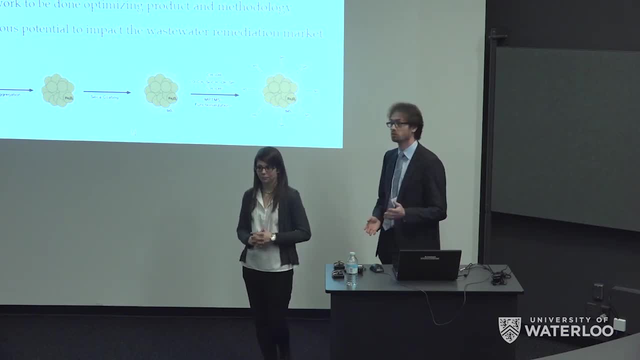 these testing. so we just wanted to be 100% certain and just do overkill- listen certain aspects. this is not new in the sense that what you're doing is new. it there are. the literature is already been talking about super parametric iron oxide coated with thiols to remove wastewater. how is what you were doing different from? 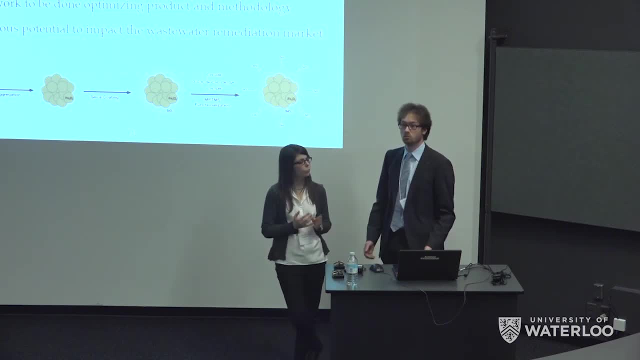 what has already been tested on it ten years now. well, what we did that was different was we used the CSAs, which are controlled sphenic acuerdoids, and these are um larger iron particles in general, like a much larger iron, so they'd have a larger magnetic moment. and so when you use a magnet, the magnet 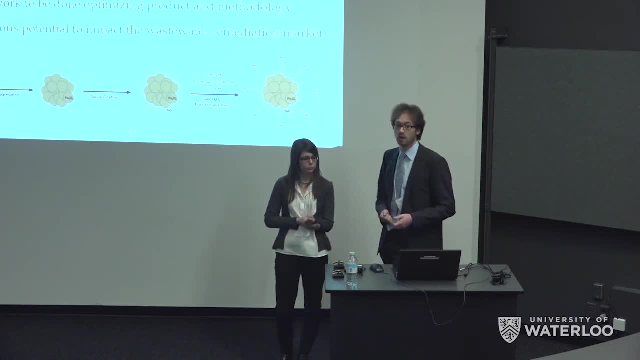 would be a lot more effective at pulling these particles of the solution, and that's what we wanted to work with. okay, so is it so what you're the spin you're putting on it? is it going to be very important for you to have a very long-term use of these anige, because you know the, the calculation? 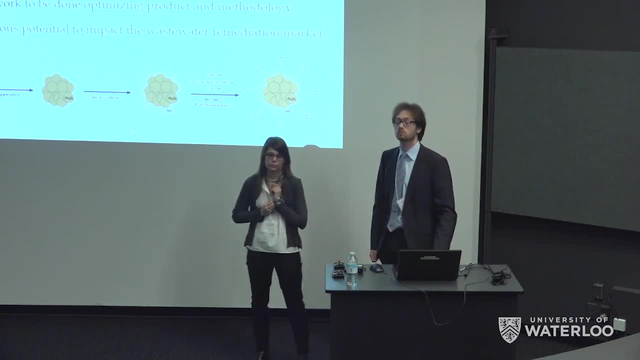 that you're putting in the process is it's not going to be very long-term use of these particles. okay, so is it? so what you're, the spin you're putting on it- is that a fairly commercial because it's a lot of energy? The spin you're putting on it is an ease of separation idea. 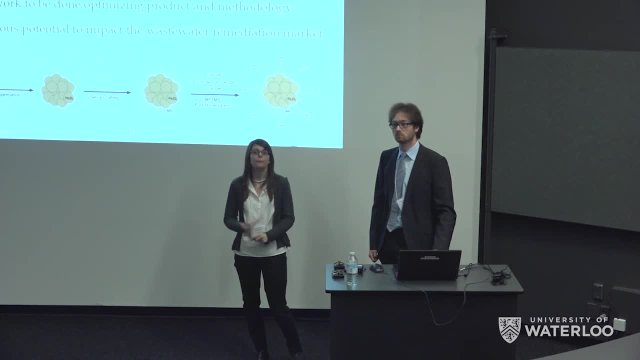 I would present. the idea of reusing hasn't been really clearly anchored in the literature, And I think this is also a couple of other things. I've seen some of it in the literature, which is why I didn't see it. Yeah, I think what you're doing here.